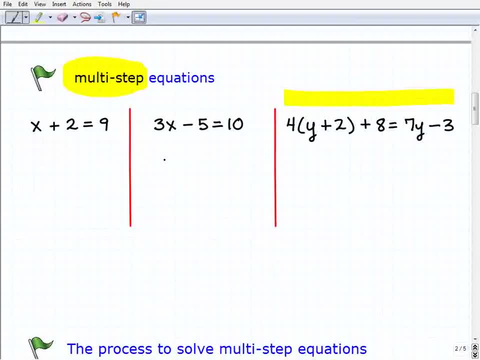 and then the second equation is a two step. So this is a good chance for you to review, and just to kind of check your understanding, Whether you've already, you know, kind of mastered these basic equations. I want to pause the video and give these problems a try. Okay, so x plus 2 equals. 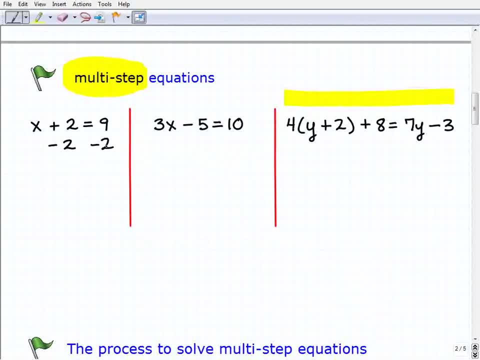 9.. So we're going to go and subtract 2 from both sides of the equation and we get x equals 7.. That was our one step to solve this equation. Okay, pretty easy, pretty basic. So hopefully most of you got this and totally understand why the 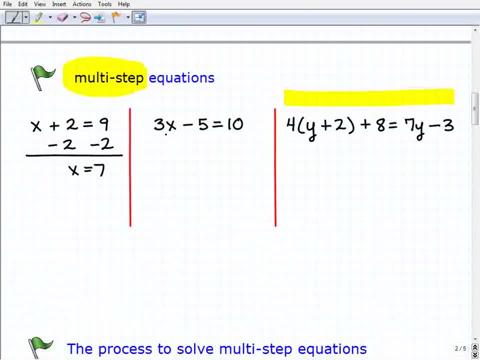 inverse operations. Now the next one is a two step equation. The first thing I'm going to do is add 5 to both sides. Okay, then I'm going to go and add down. I'm going to get 3x equals 15.. And then my second step is I'm going to divide both. 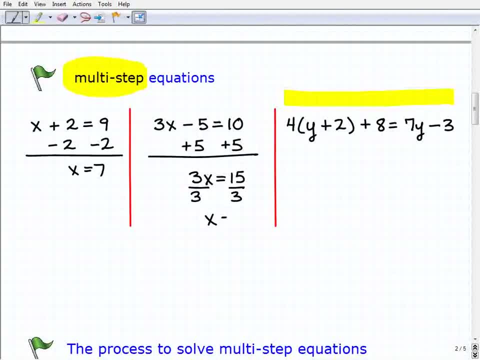 sides of the equation by 3. And then I'm going to get x equals 5.. Okay, so if you got these both of these equations correct and you understand them, and there's no problems, then you're really, really you're ready to take on multiple step equations, Because multi-step equations 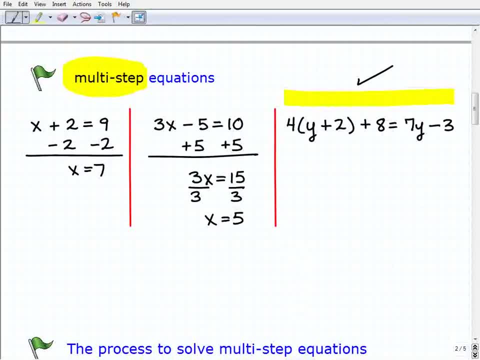 are essentially just a series of one and two step equations all kind of wrapped up into one equation. Now, the two things you're going to need to solve a multi-step equation are: one- you're already going to have to know how to solve these one and two step equations, as we already talked about, And the 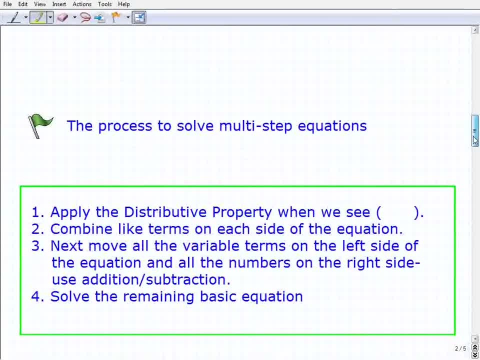 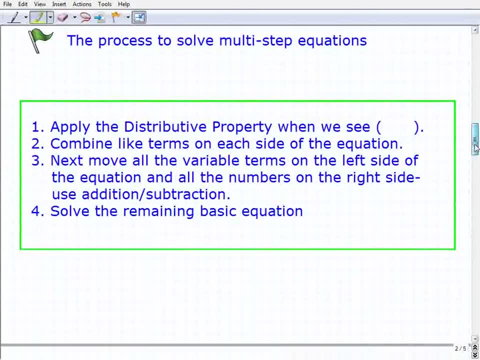 second thing is you need a kind of a general set of directions, a general set of rules, And that's what this is here. Okay, so you might want to go and write this down and put this in your notes, And then we'll actually take a look at a couple examples. 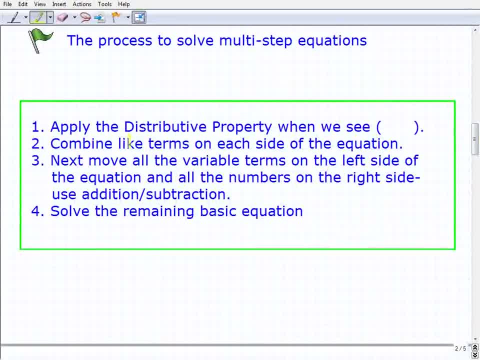 and see how to apply this procedure. Okay, so the first thing you're going to do is you're going to apply the distributive property when you see two parentheses and a number outside of it- And I'll show you here in the example what I'm talking about- Then, next, you're going 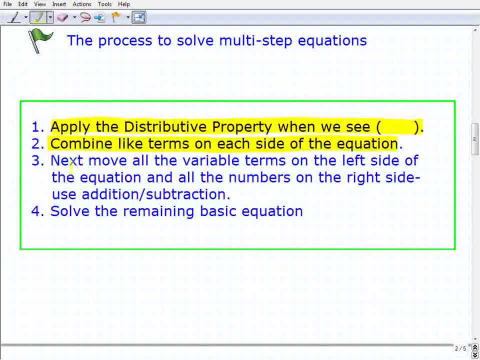 to combine like terms on each side of the equation. Okay, then you're going to move on and you're going to put all the variable terms on the left hand side of the equation And all the numbers on the right hand side, using addition and subtraction inverse. 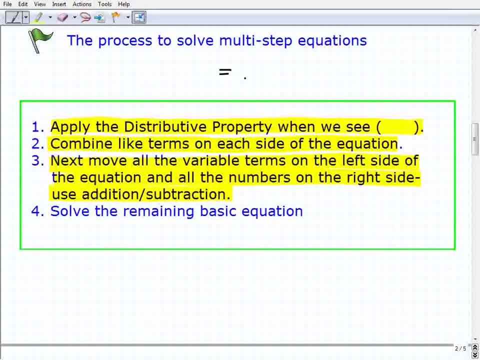 operations. Remember, we want what we're trying to do when you solve a, when you're solving an equation, is to get all those variables on the left and all the numbers on the right. Okay, so that's what we're talking about in step three. Then, lastly, after step three, 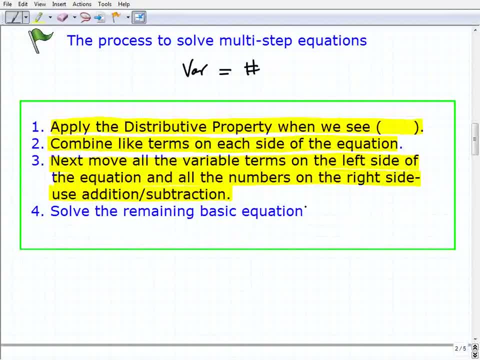 what you're going to be left with is a basic one step equation. So you're just going to solve that basic equation and you'll get your solution to your multi-step equation. So let's take a look at a couple of examples. Okay, so first thing is we're going to go ahead. 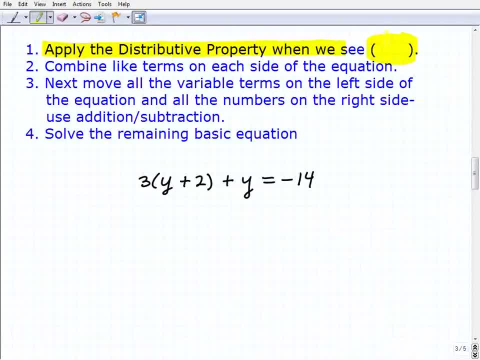 and apply the distributive property when we see parentheses, and we see parentheses with the number outside of it. So, in other words, this is a distributive property situation. Okay, so you have three parentheses: Y plus 2.. Now let me emphasize the distributive property. 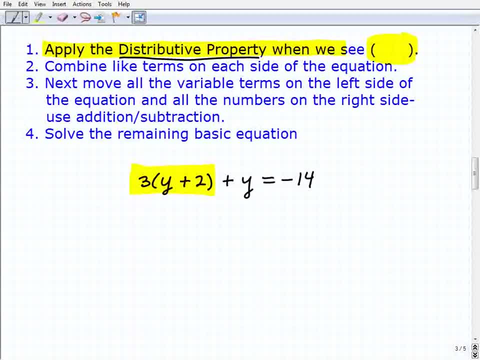 because oftentimes, when students struggle with these multi-step equations, it's because they don't really understand the. So go back and review the distributive property. if you need to do that, Okay. if you're. you know when you're doing these problems and you're seeing that you're getting them wrong. 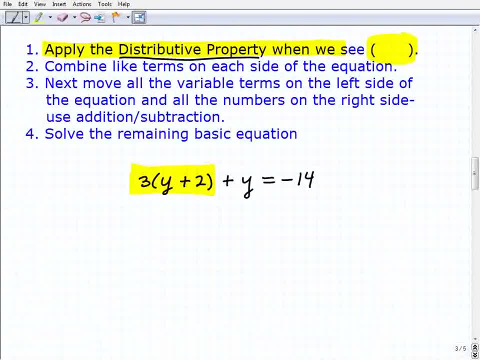 because of the distributive property. obviously that's an area you want to go back and review. Okay, so the first thing I'm going to do is apply the distributive property. So I've got 3 times y plus 2 plus y equals negative 14.. 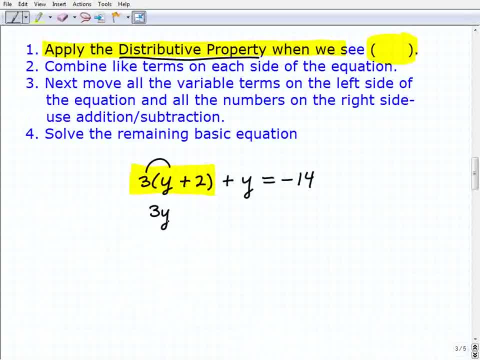 So that's going to be 3 times y. Okay, this is the distributive property plus 3 times 2, which is 6, plus y equals negative 14.. Okay, so notice how I rewrote the equation right underneath it. 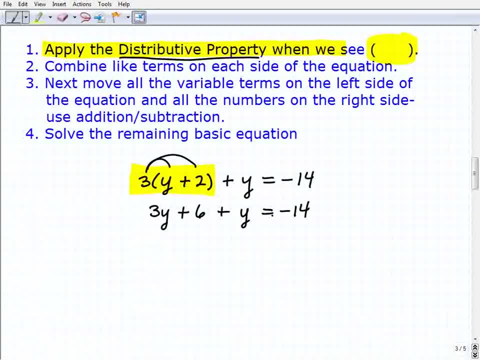 but this time I used the distributive property to rewrite it. Okay, so that's step 1.. Okay. step 2 is to look for opportunities to combine any like terms. okay, on either side of the equation. So we want to look at the left-hand side independently. 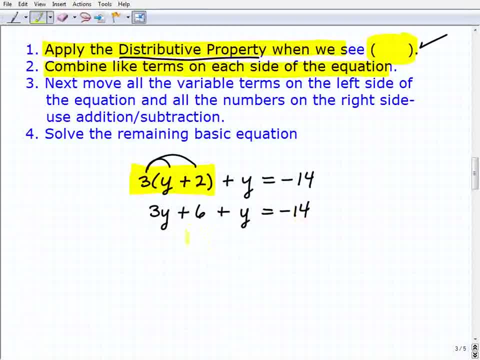 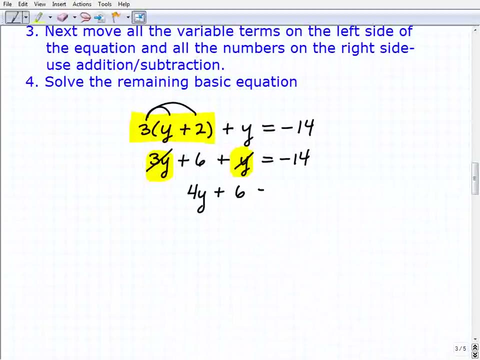 Of the right-hand side and just look for like terms. Okay, so, do we see any like terms here? Well, 3y and y are like terms, so we want to combine them. Okay, so 3y plus y will give us 4y plus 6 equals negative 14.. 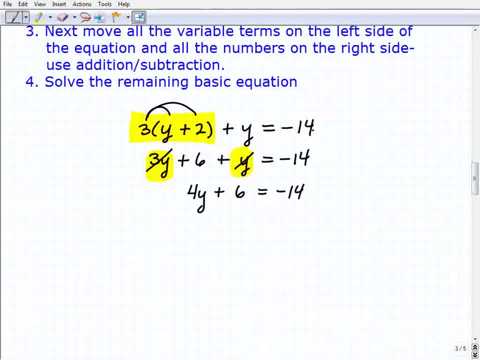 Okay. so if you notice, here, what I'm doing is I'm rewriting the equation over and over again, but each time I rewrite it, I'm making it simpler. Okay, that's the whole idea. That's the whole idea behind solving these multiple-step equations, and you're showing all your work. 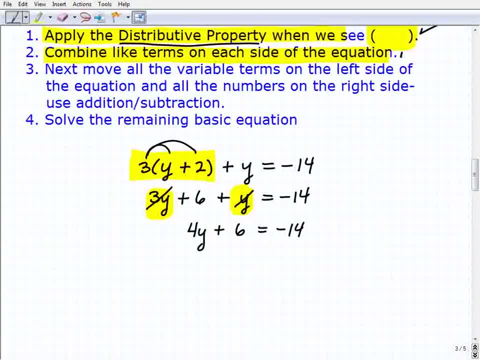 Okay. so what I did there was I combined like terms, okay, on either side of the equation. In this case, it was only like terms on the left-hand side. So next, okay, I'm going to move all my variable terms to the left-hand side. 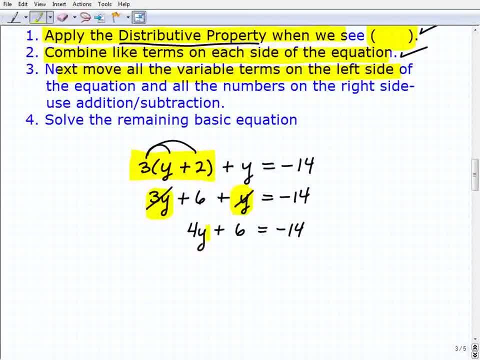 So if I look here, my variable term is already on the left-hand side. There are no more variable terms. But I also have to move all my numbers. So I'm going to move all my numbers to the right-hand side and I'm going to use addition and subtraction inverse operations to do that. 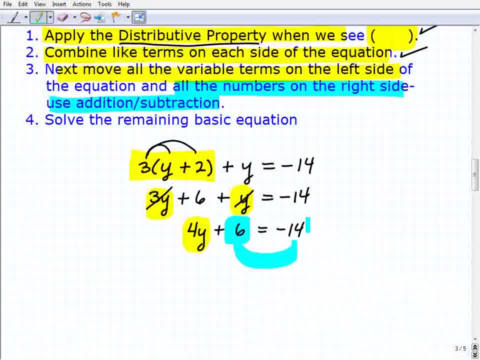 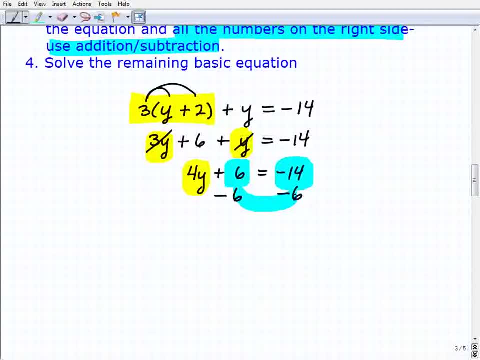 So here I have a 6.. I don't want that 6 there. I need to get that 6 over to the right-hand side with that negative 14.. So I'm going to subtract 6 from both sides of the equation. 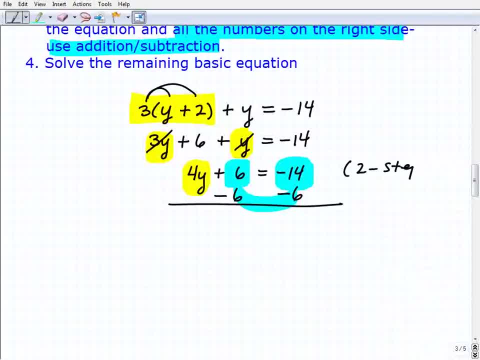 Now, at this point, this is a simple two-step equation, Okay, so hopefully you've noticed that 4y plus 6 equals negative 14.. Really, at this point forward, you can go ahead and just take the steps to solve it. 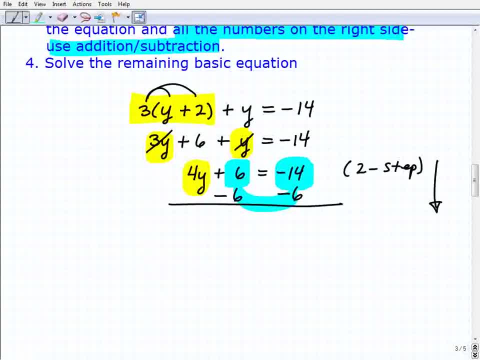 It's a simple two-step equation and get your solution, But we're just going to go ahead and follow this general procedure that I gave you. So, subtracting 6 from both sides, I get 4y equals negative 20.. Okay, and then I'm left with this basic equation. 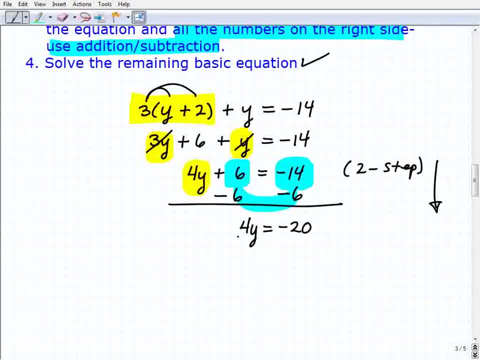 So I'm going to go ahead and solve that. 4y equals negative. 20 is a basic equation, So I'm simply going to go ahead and divide both sides of the equation by 4, and I get y equals negative 5.. 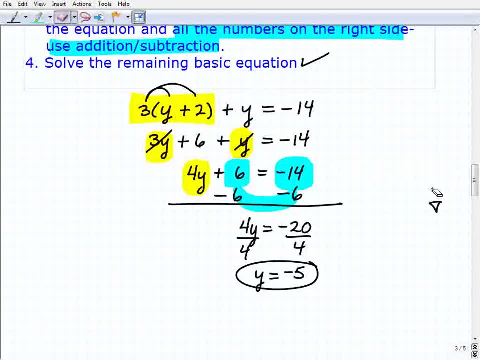 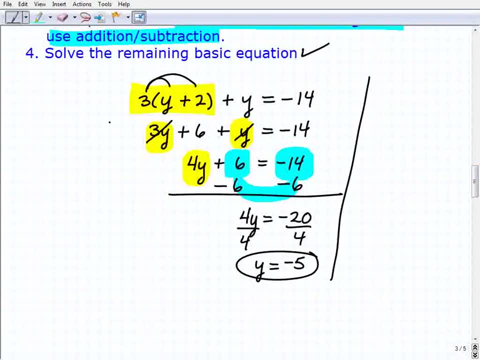 Okay, So that's it. This is how you solve a multiple-step equation. You're going to use these steps as a general guideline and just kind of walk it through. But notice the way I'm working. Okay, Nice and neat. I'm showing all my work and I'm essentially rewriting the equation simpler every time. 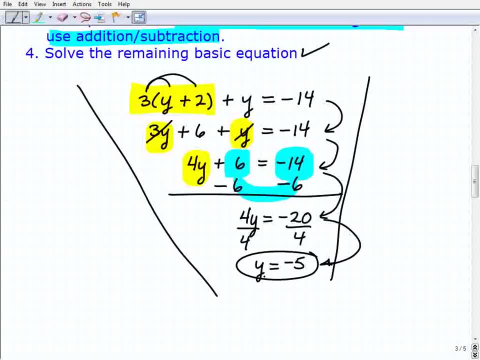 until I get to the most simplest form of that equation, which is the solution: y equals negative. 5 is the simplest form of this equation right up here. Okay, All right, so let's go ahead and try another problem. So here is our procedure again. 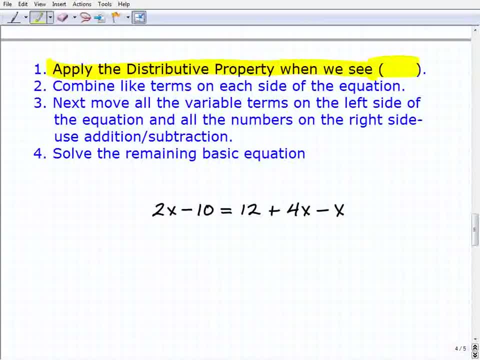 So the first thing is, I'm going to apply the distributive property when we see parentheses. So in this case, do we see any parentheses, any situation where we have to apply the distributive property? No, Okay, so you're not always going to have to do these steps. 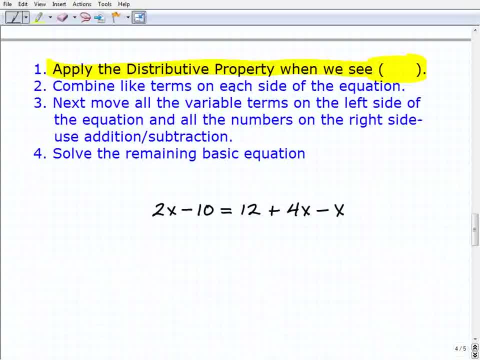 You'll do them if you in fact see them in your multiple-step equation. So that's done. So now the second thing is: I'm going to combine like terms on each side of the equation. So I'm looking on the left-hand side. 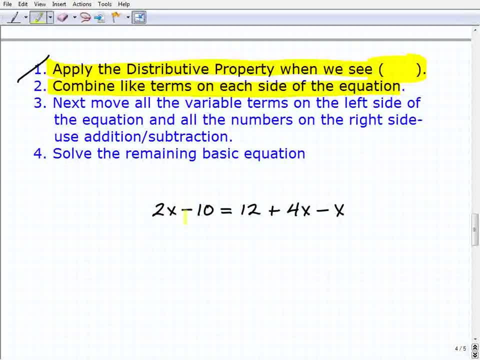 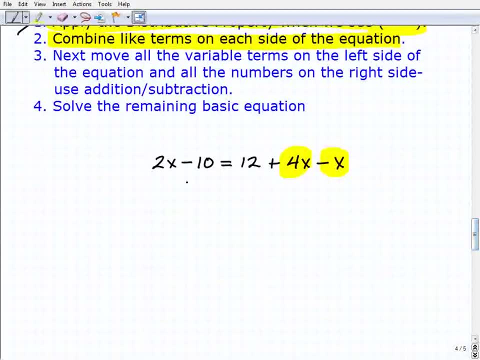 I've got 2x minus 10.. There's nothing to do there. On the right-hand side, I have 12 plus 4x minus x. So these two are like terms, So let's go ahead and combine those. So I'm going to rewrite the equation. 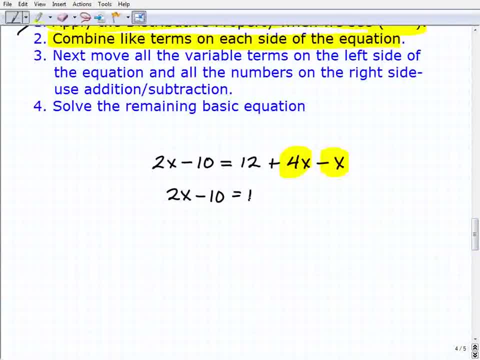 2x minus 10 equals 12 plus. Now you've got to know how to combine like terms. Another area if you're weak and you want to review. So 4x minus 1x is going to be 3x. 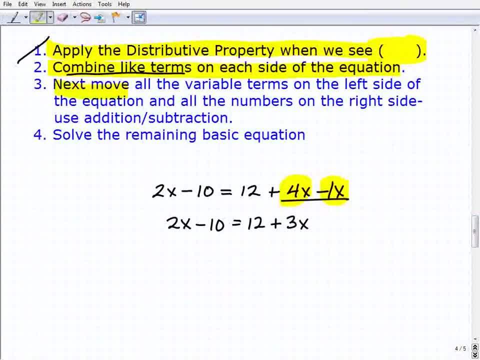 Okay, Our next step is we're going to move all the variable terms to the left-hand side. Okay, so, therefore, this 3x I've got to move over to the left-hand side And then I'm going to have to move all my numbers to the right-hand side. 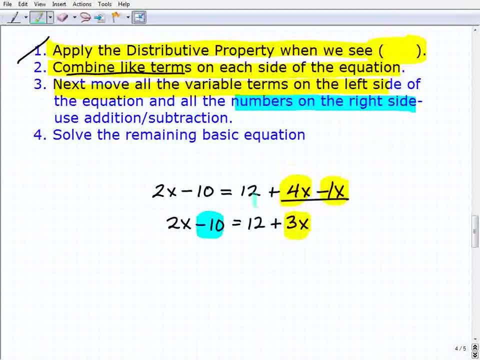 So this negative 10, I'm going to have to move to the right-hand side. So let's go ahead. Let's go and handle the 3x first. Let's get that over to the left-hand side. So I'm going to subtract 3x on the right-hand side here. 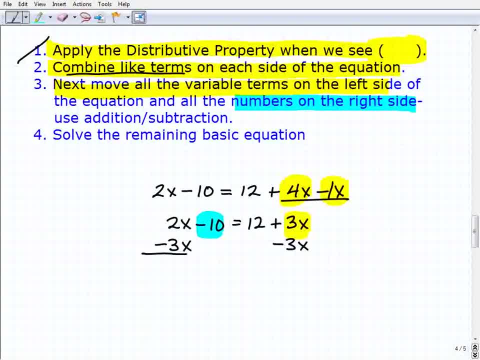 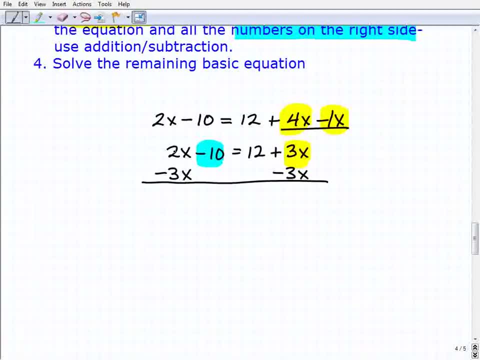 Okay, but I also have to subtract 3x on the left-hand side and notice how I'm lining up my variable terms. Okay, so, rewriting this equation, I want to get negative. 1x minus 10 equals 12.. Okay, but now I still have to take care of my number. 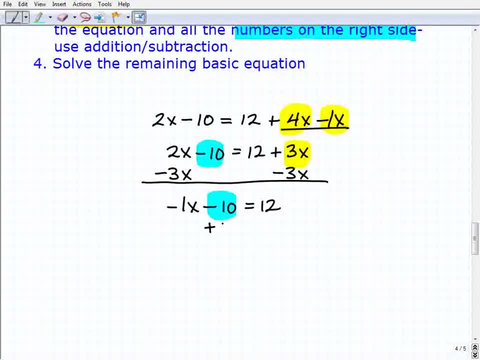 I have to move it all to the right-hand side, So I'm going to add 10 to both sides of the equation. These are just inverse operations. We talked about this way back in one step equations- how to move numbers or variable terms to the left or right-hand side. 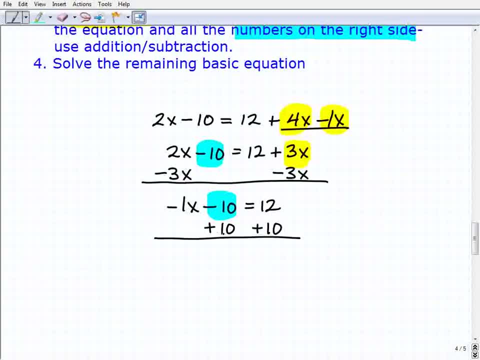 Okay, so now I'm going to add 10 to both sides of the equation. Okay, all right, so I'm going to go ahead and add 10 to both sides of the equation. I'm going to get negative. 1x equals 22.. 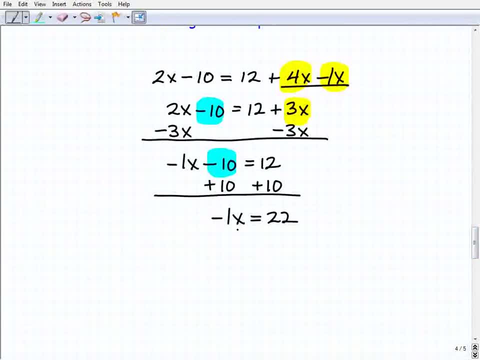 All right, so I'm left with a basic one-step equation. So to solve for x, all I got to do is divide negative 1 by both sides of the equation. I get x is equal to negative 22, and that's it. 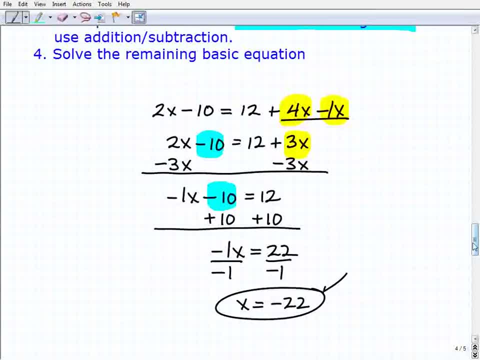 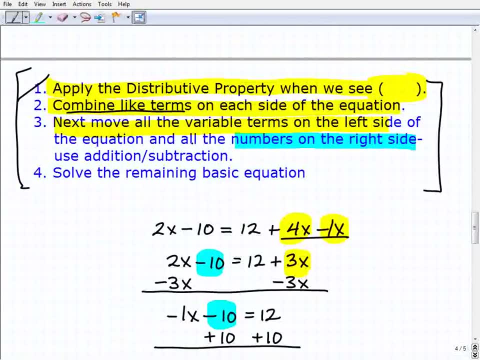 Okay. so once again, you know you use this procedure as a general guideline. Okay, not every single step is going to apply and every step is going to be a little bit different than maybe your previous problem that you did. But if you use this as in kind of like step-by-step order, you should have no problem solving these multiple-step equations. 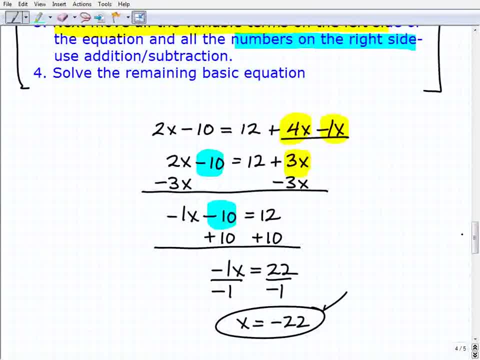 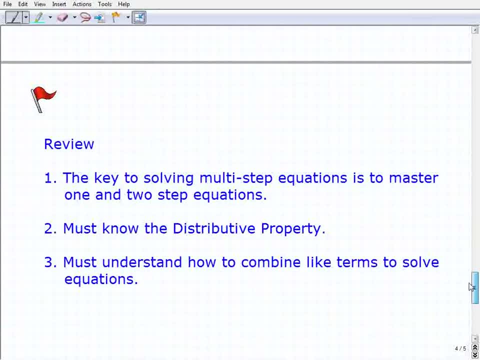 Of course you want to practice this, Then after a while, it's just going to be kind of become second nature. All right, let's go ahead and wrap this up So in review. the key to solving these multiple-step equations is to master the one. 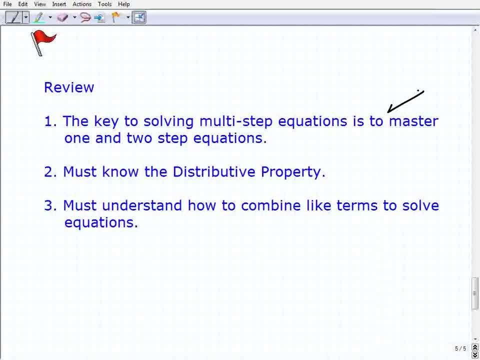 It's two-step equations. Okay, you have to have that down before you tackle multi-step equations. You also really have to be an expert at the distributive property and you have to know how to combine like terms. But if you know how to do all three of these things, then you'll know how to handle these multiple-step equation problems. 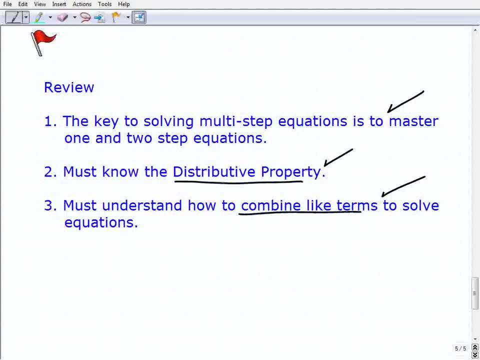 Okay, so you definitely want to practice this. Keep working hard. We'll see you soon.